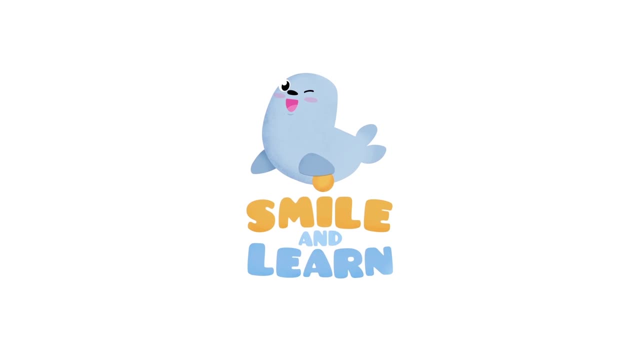 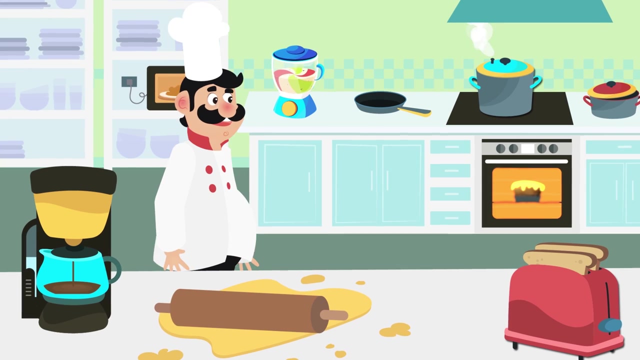 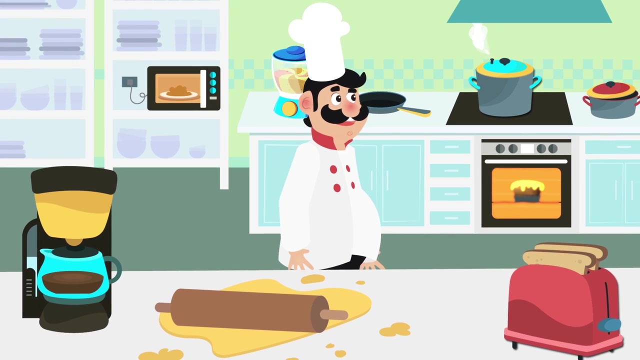 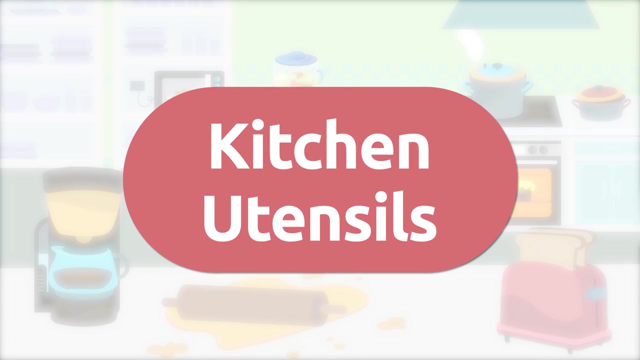 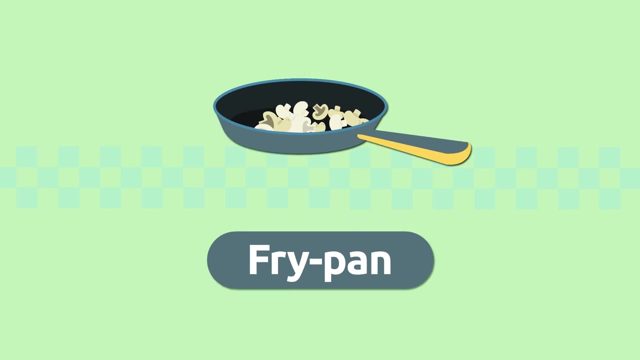 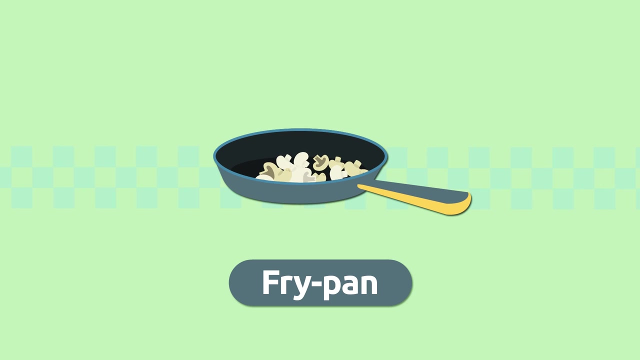 Smile and Learn. Hello friends, Today we're visiting the kitchen of a great chef to learn many words about this place. Are you ready to discover which utensils and electric appliances we use in the kitchen? Here we go. Frypan: A frypan is a kitchen utensil we use to fry foods. Careful not to burn yourself, Frypan. 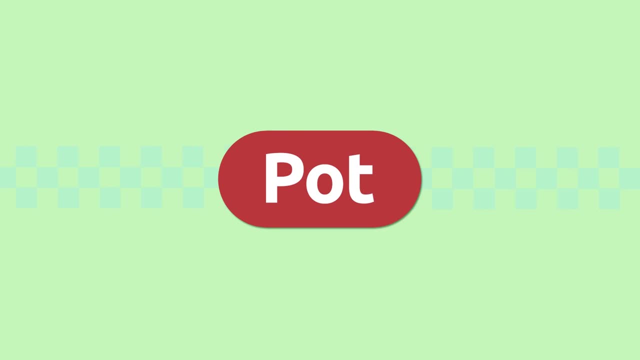 Pot: A pot is a round container with two handles. We use pots to cook food. Mmm, smells good. Pot Pressure cooker: We use a pressure cooker to cook food quickly using water. steam Pressure cooker. Blender: A blender is an electric appliance we use to mix and blend foods. My fruit smoothie is ready Blender. 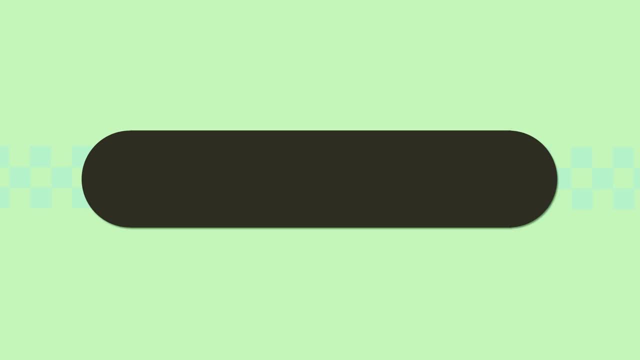 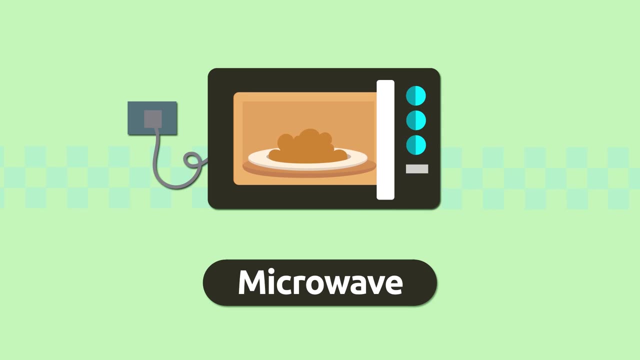 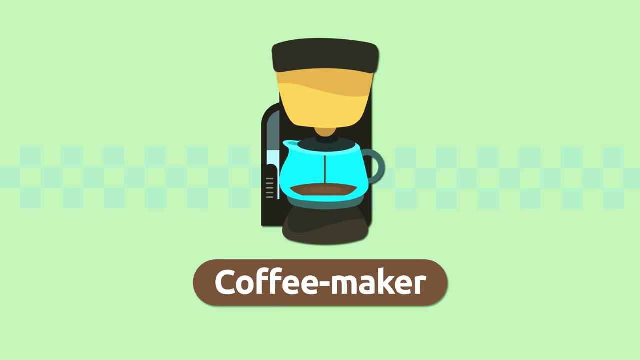 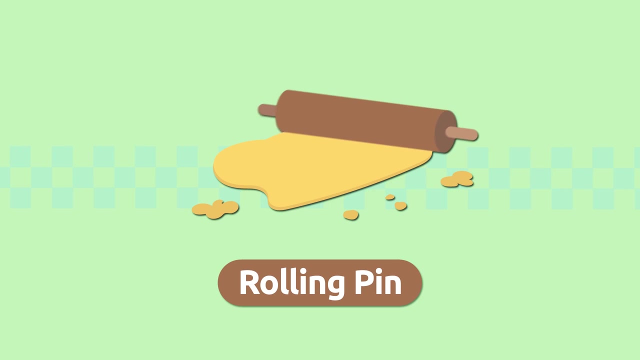 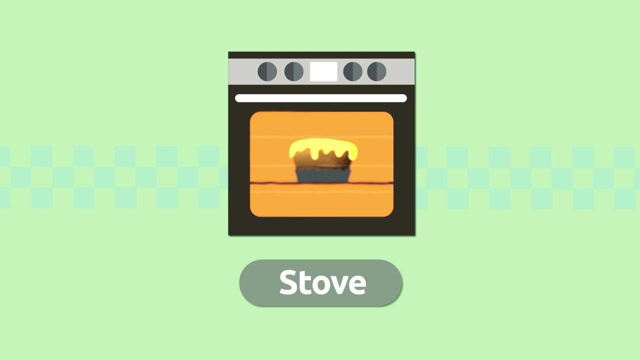 Microwave- Microwave: A microwave is an electric appliance we use to warm up food quickly. Microwave Flour dough, for example. rolling pin toaster: a toaster is an electric appliance we used to toast bread, hurry, pull them out. toaster stove: a stove is an electric appliance that provides heat for cooking different types of food. the cake is: 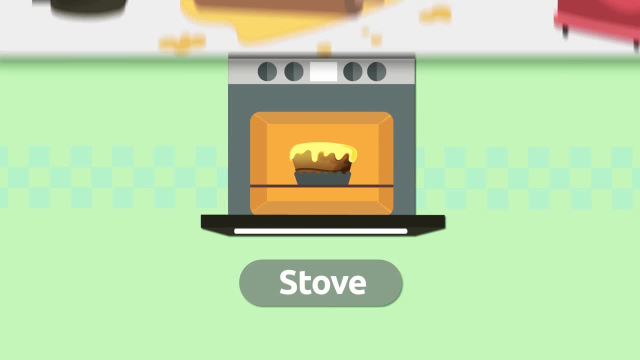 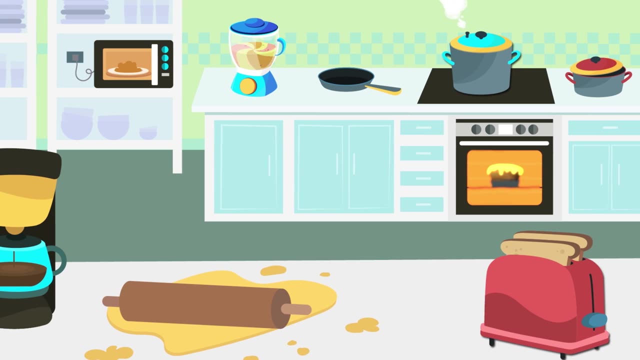 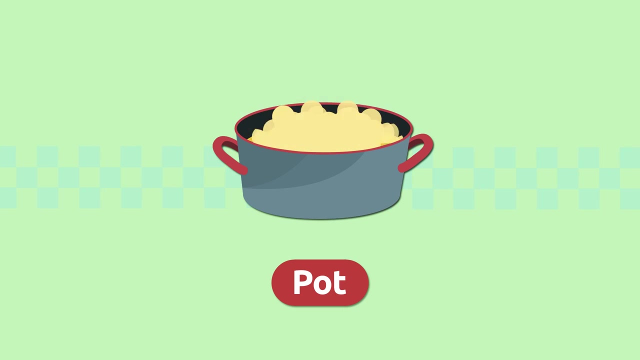 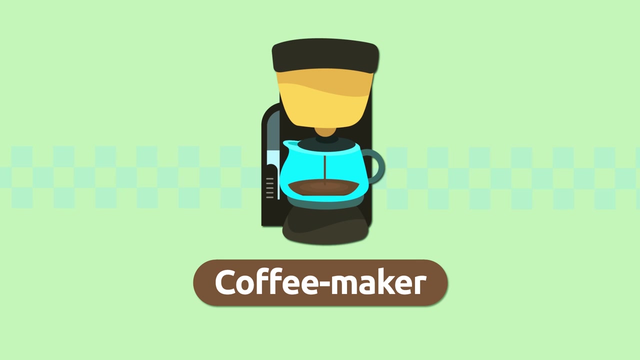 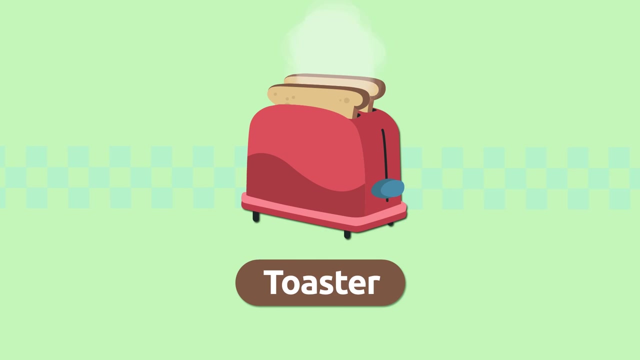 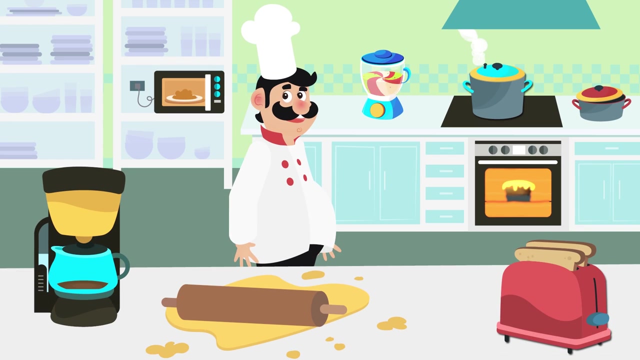 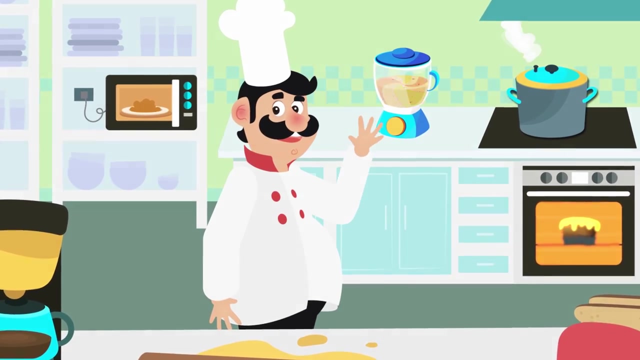 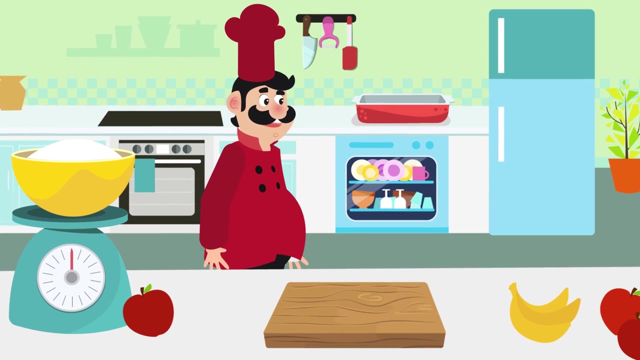 ready stove. can you remember all the words we learned today? let's recap them: frypan, pot, pressure cooker, blender, microwave, coffee maker, rolling pin, toaster stove. thank you, chef, for letting us visit your kitchen. we had a great time see you around. today. we're back in the kitchen of our friend the great chef. 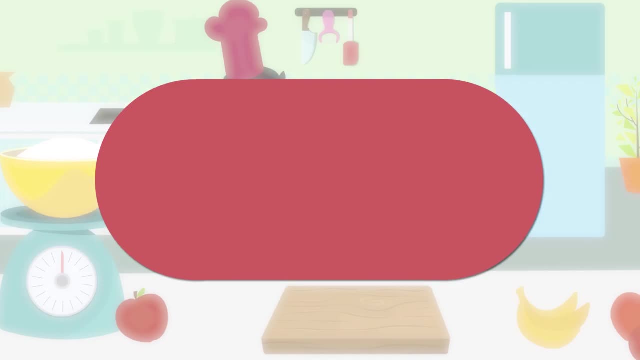 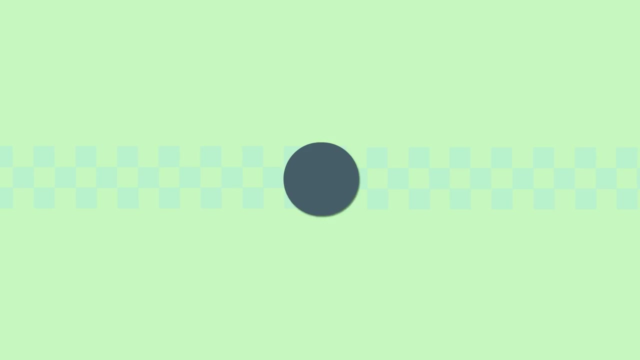 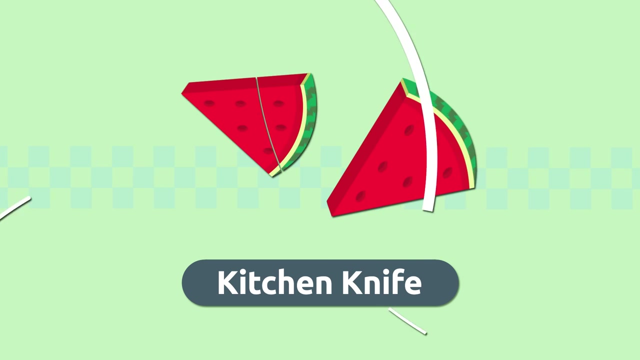 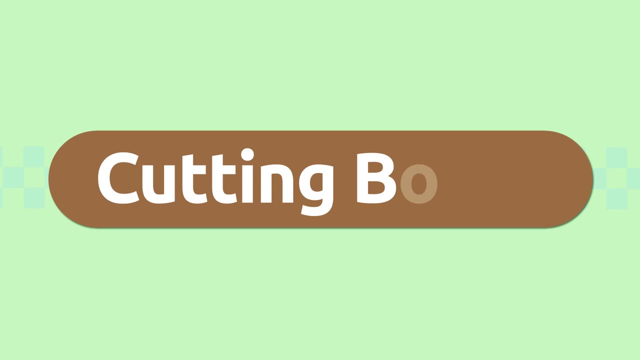 where we're going to learn tons of new words about kitchen utensils. are you ready? kitchen knife? we use the kitchen knife to cut and slice all types of foods. careful not to cut yourself. kitchen knife cutting board: it's a flat surface that you chop food on. 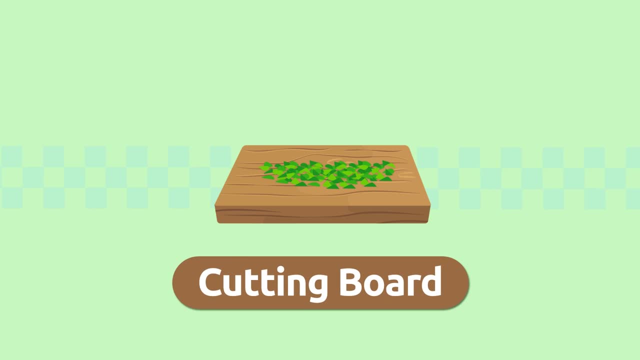 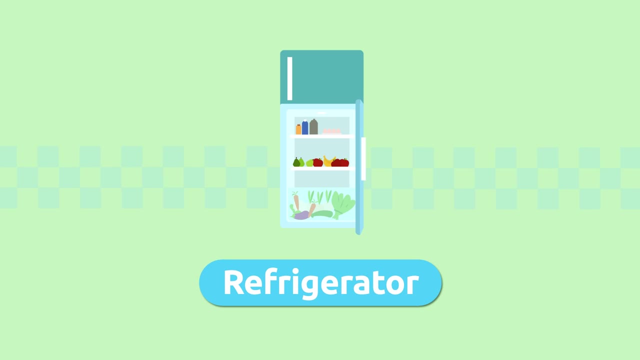 can be or plastic cutting board refrigerator. we put fresh foods in the refrigerator to keep them cool. refrigerator freezer: please turn. the freezer is very low. this freezes foods and helps to preserve them for a very long time. dishwasher is usually part of the hoist fix. einen cattle setter can also be chicken memorable food. cut Bench mineraal. 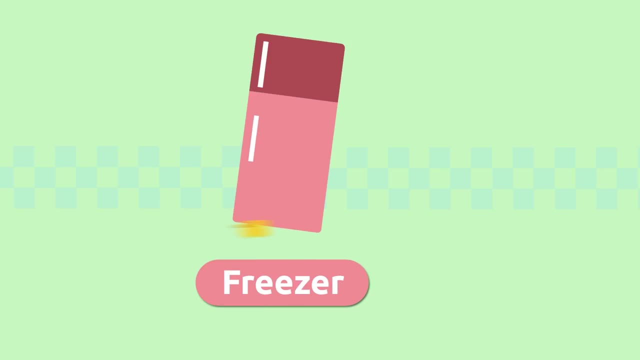 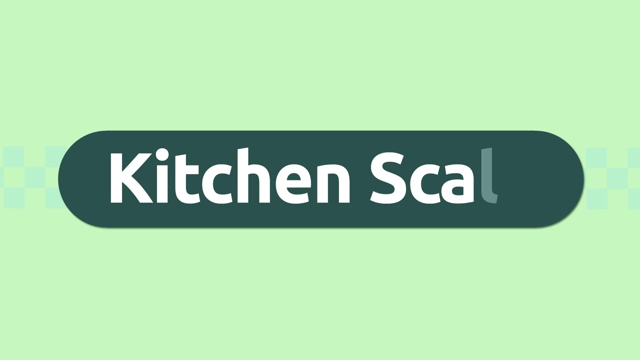 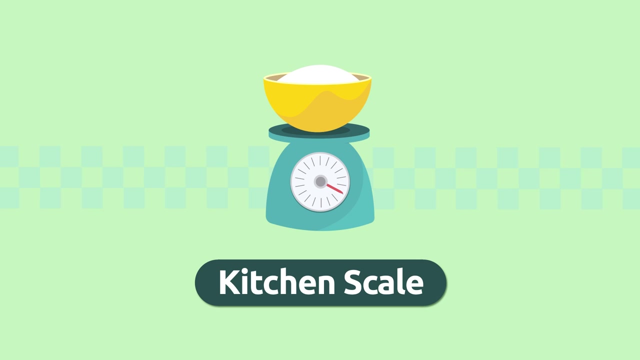 of the refrigerator freezer platter. a platter is a very large dish we use to put food on. then we take the platter to the table and serve the food platter. kitchen scale. a kitchen scale is the device we use to weigh foods. i'm going to need 10 ounces of flour for this cake recipe. 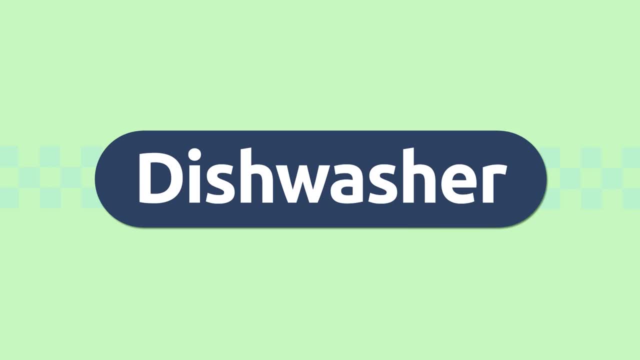 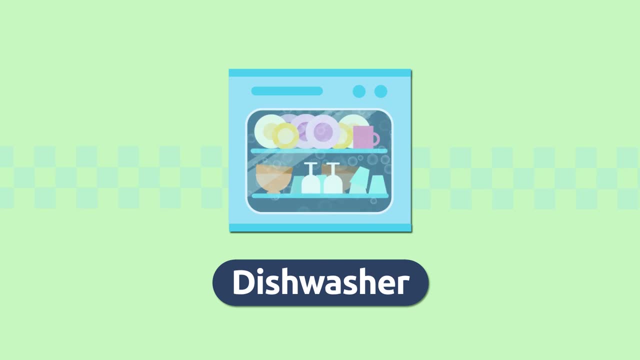 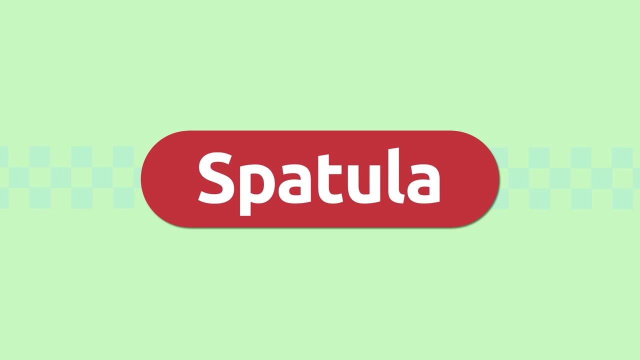 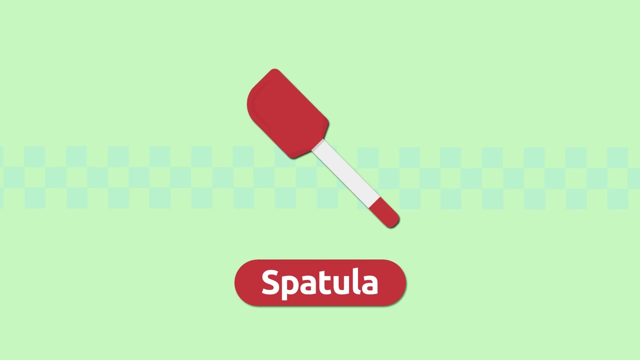 kitchen scale dishwasher. a dishwasher is an electric appliance we use to wash all kitchen utensils automatically. dishwasher spatula: a spatula is a small palette we use to spread frosting on a cake, for example. spatula peeler: a peeler is a special knife we use to peel fruits and vegetables more easily. 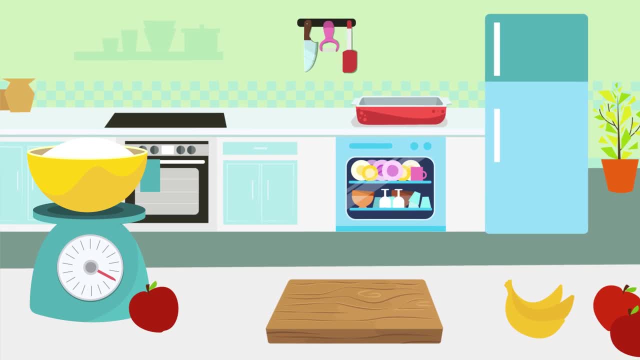 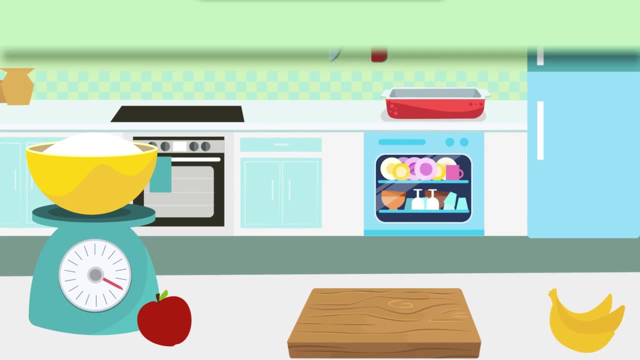 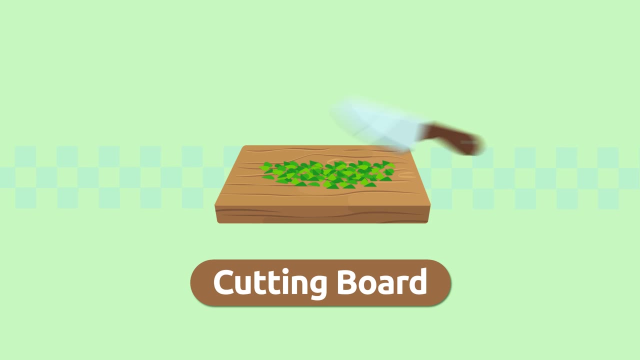 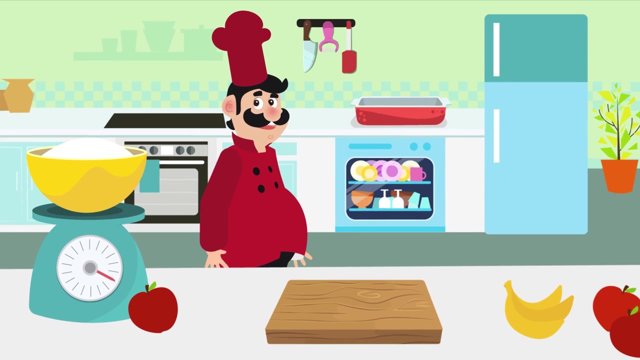 peeler. can you remember all the words we learned about electric appliances and kitchen utensils? let's recap them: kitchen knife, cutting board, refrigerator, freezer, dishwasher platter, kitchen scale, dishwasher, spatula, peeler. thank you, chef, for showing us all these kitchen utensils. see you in the next video. bye, bye, friends. 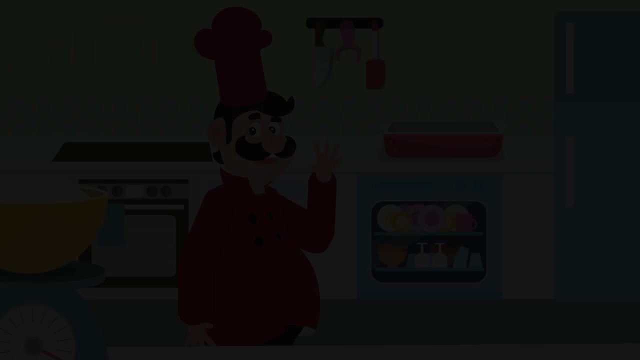 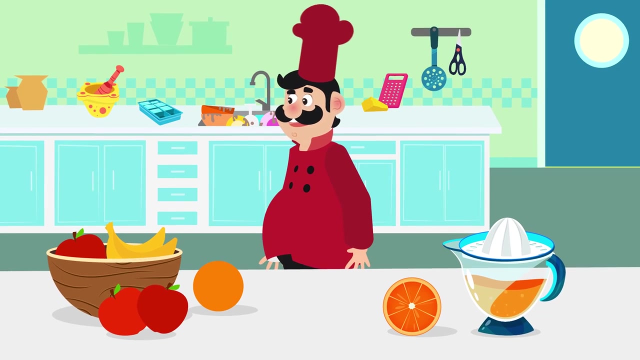 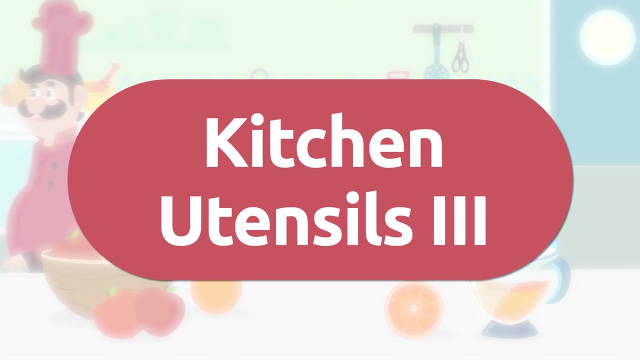 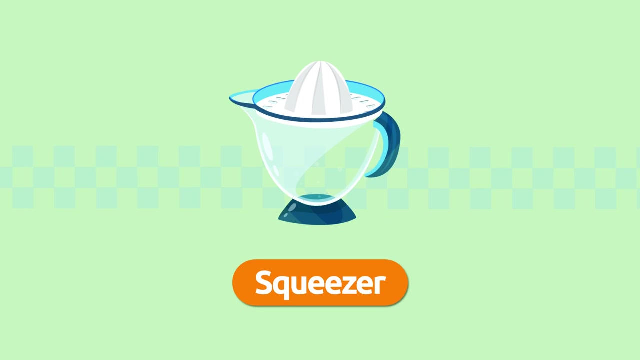 hello friends. welcome to the chef's kitchen. he's our great friend. this is our last video where we'll learn about kitchen utensils. have you watched the other ones? here comes the third video: squeezer. we use the squeezer to squeeze juice from fruit like oranges or lemons. 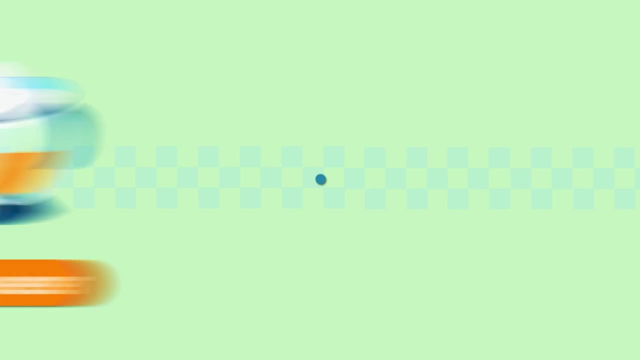 squeezer quake, squeezer squimer. we use the skimmer to stir or scoop foods out when we fry them in the fry pan. skimmer squ, salts, skimmer itty. We use the grater to shred or grate foods into fine pieces, like cheese, for example, that we add on pasta.